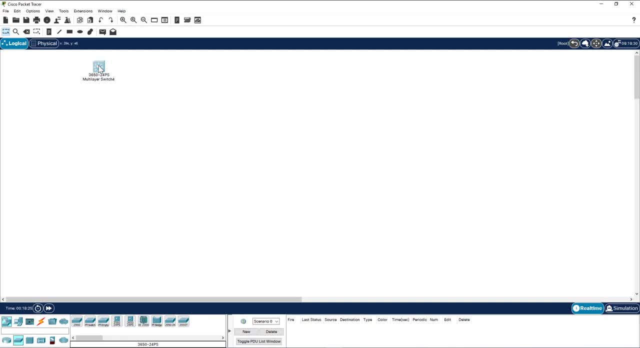 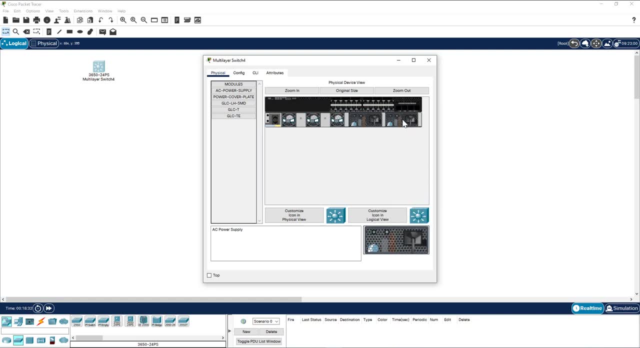 And this is a 3650 multi-layer switch. It is a modular switch, So you have to insert the power To the device, Otherwise you are not able to turn on this device. Also, you have to install the uplink module here. So you go here and select here. 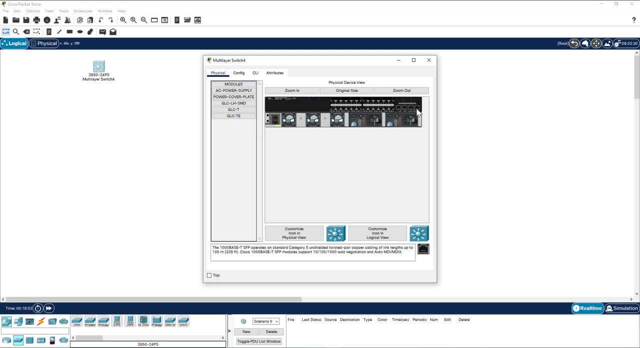 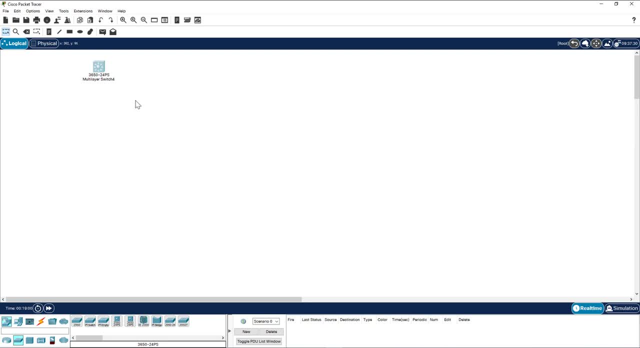 Just track it and bring it here. So you have all the uplink ports enabled. I am going to need two more switches. So what I am going to do is I am going to select this device And I'm going to use a copy, Control C, and I'm going to paste twice. So I will get three more devices, two more device. So I have two switches. 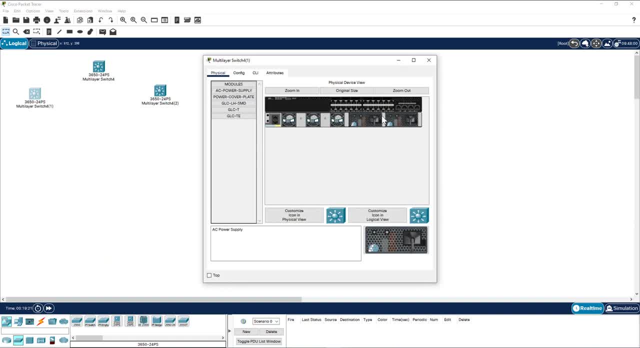 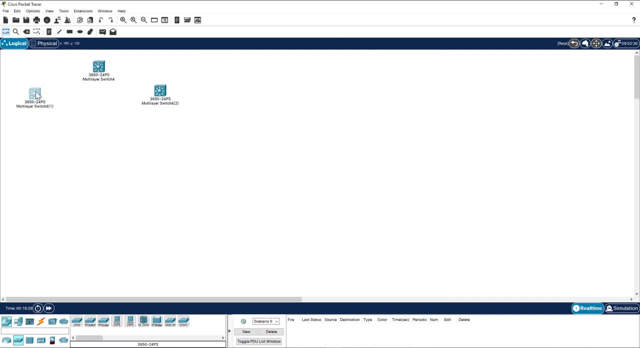 So this way I do not have to pre-configure these devices with the power and uplink ports. All have been copied from this configuration And now I'm going to place two axis layer switches. I go to 2920.. 6960- click here and click this one. and click here and click this one. but i can place more. 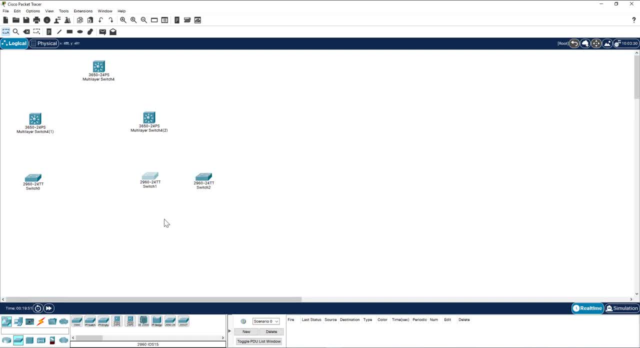 access switches here, if i want. also, you can copy and paste, like i showed before. so i'm going to put two more here so it looks nice from the topology point of view. all right, now i have to choose the cable type. so come here to the cable type and select automatically. choose connection. 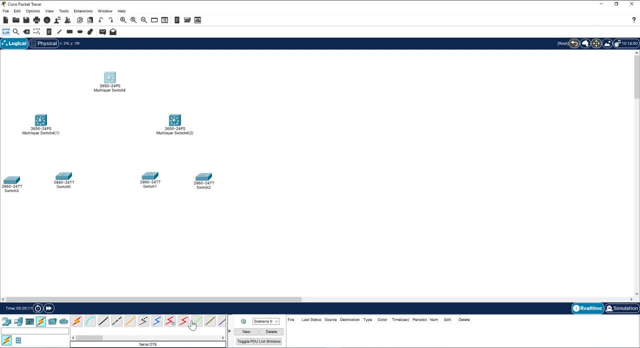 type. otherwise you have to select those cable individually appropriately. that is a little tough. so you select this one, it will choose the cable type automatically. so i come here and i'm going to click this one click here, i'm going to just randomly click all of them and i'm 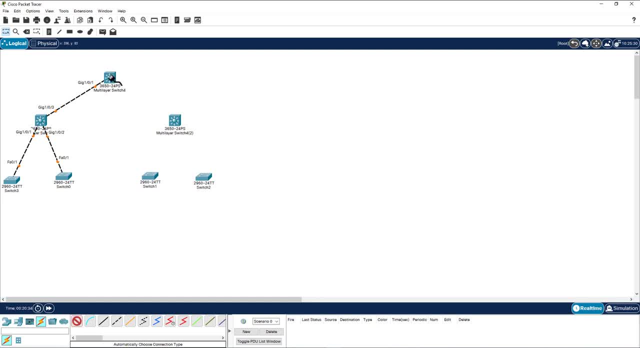 going to select the right port later on. click here. click here. click here, so now you can select the right ports. i supposed to be connecting this to my uplink port for this one, so you always start from the top. click on the device. you select this port. this is uplink port and go here. click on this icon. 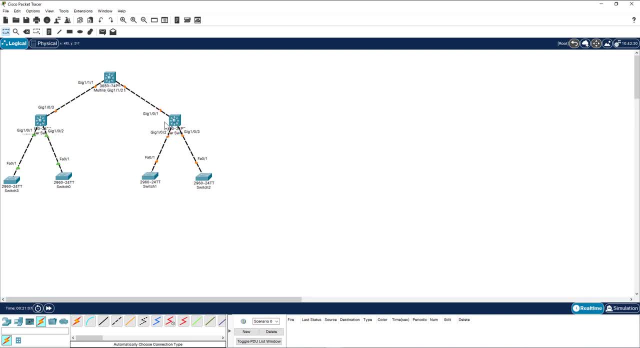 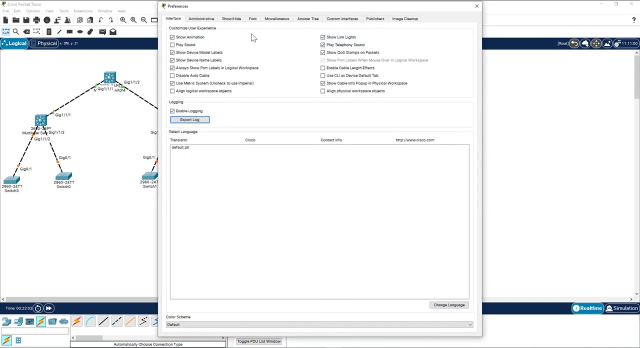 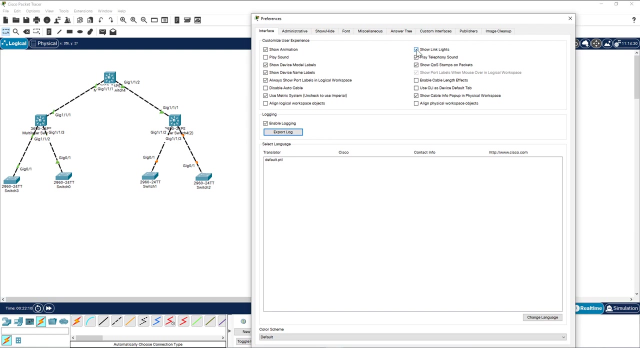 here, here, and you can see that i have selected the right port. and now you can see this is the one that i have selected. okay, so you can see the link light is gone. so make sure the link light always selected. if i select unselect this one, all the link lights are gone. if you don't have a link, 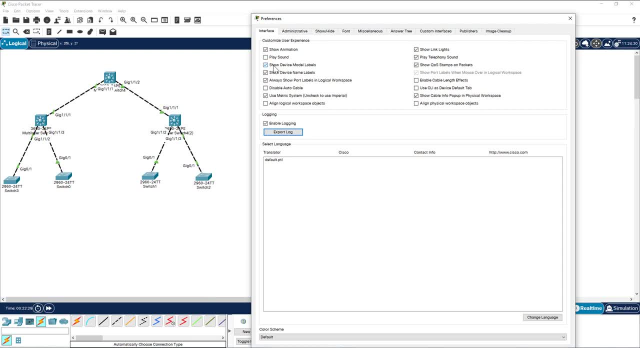 light. you don't know what stage this link are at right now, so make sure you select this one. so you know this link has not come up now. it's up and running, okay, so i'm going to go ahead and uncheck this one. all the model labels are gone. so if you look at, 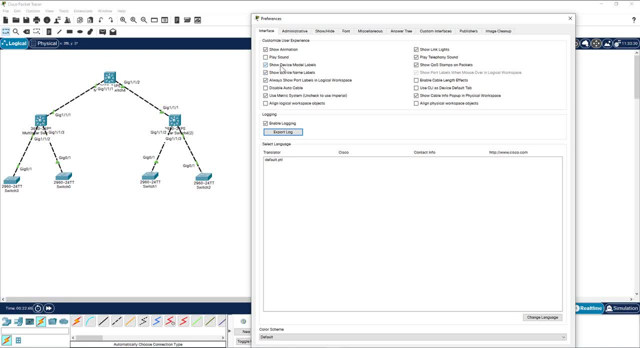 here. it is telling you what kind of switch this is. so you can keep it or you can uncheck it. i normally uncheck it because i know what switches i am using. so i'm going to uncheck this one, but i'm going to show the device label. but if you are labeling the switch individually, you don't need that. so what i'm? 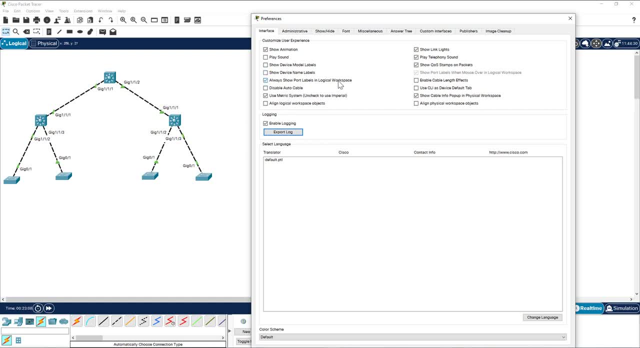 going to do is- i'm going to check this one also, but i'm going to make sure always show port label in the logical workspace. this is it's a very useful feature, because you need to know what ports you are working with, so i will always leave it on this port label. now i am going to go to. 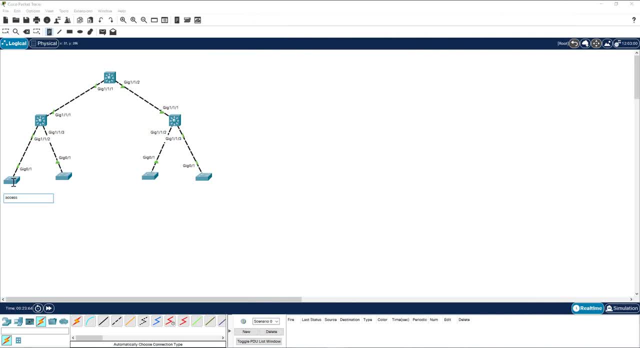 my label here: click here and you can label the switch: access, dash one and you can select this, select this one and you can copy paste and i am pasting couple of times so i can grab it and then i can change the label here: dash- access to access three. 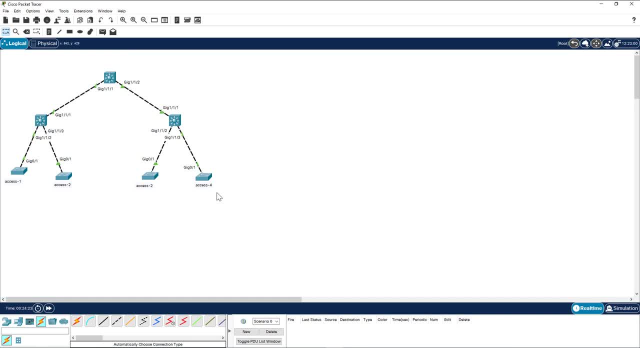 access four and you can do the same thing here. i'm going to paste, paste it here. i'm going to grab it to here. i'm going to name this radial one, radial two, and i'm going to copy and paste here. uh no, it is copying everything. so i come here, click this one, delete, because it will be deleting. 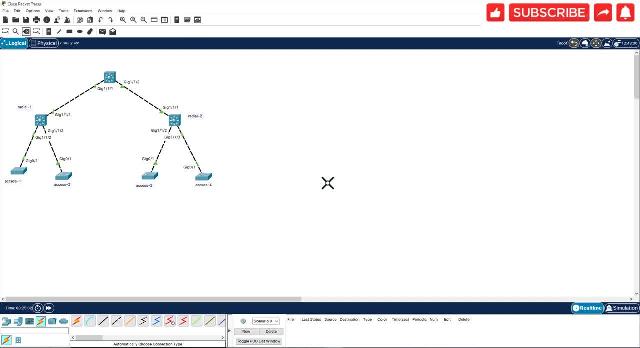 the selected grayed out one, so it's deleting everything and then hit escape. and now i'm going to just select this one. copy paste. so make sure what you are copying. so i'm going to say core. so now i have labeled them all. however, it is not labeled inside the switch. you have not changed. 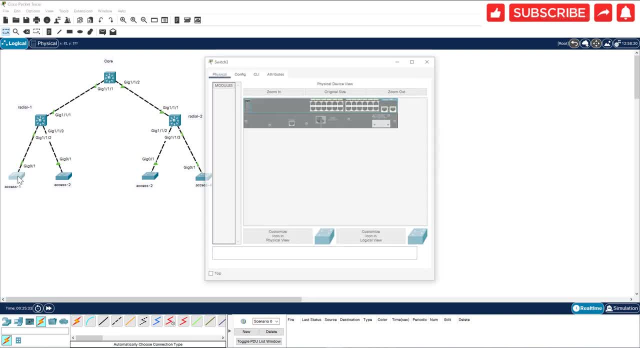 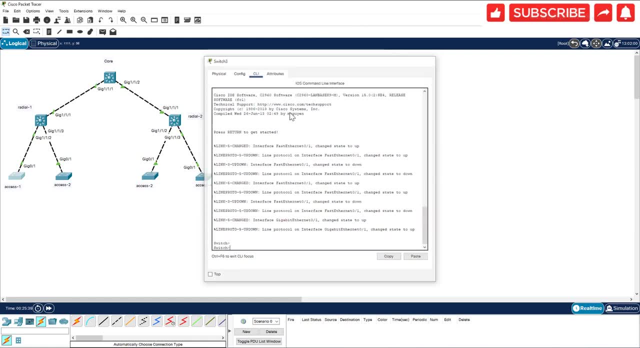 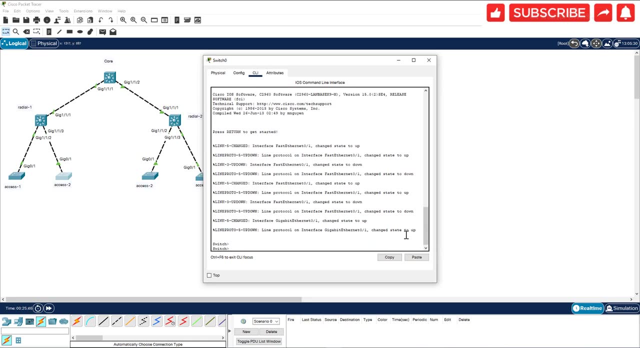 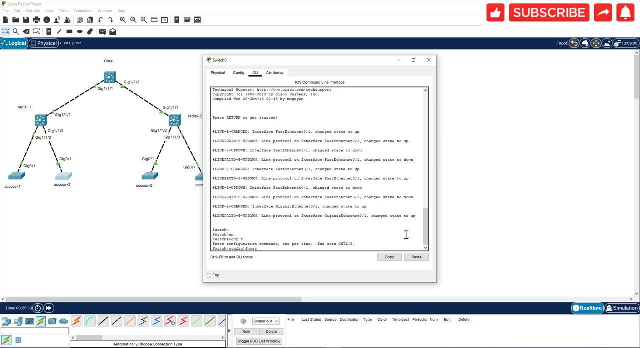 the host name of the switch. so when you click here, go to cli, it is going to show you switch. so it's going to do the same thing for this one. even though you labeled outside, you have not named those devices. so i'm going to go to enable conf t host name and i'm going to say access. 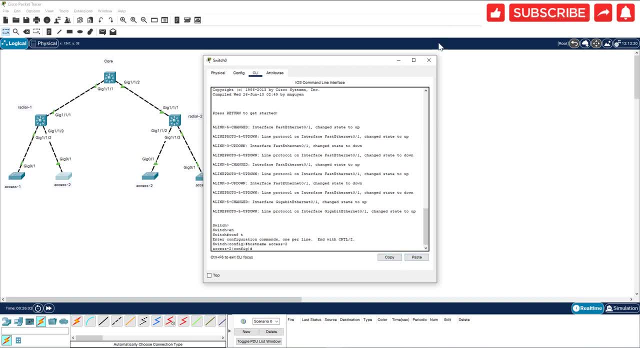 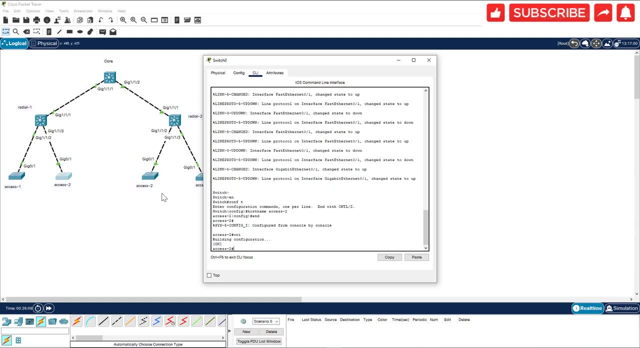 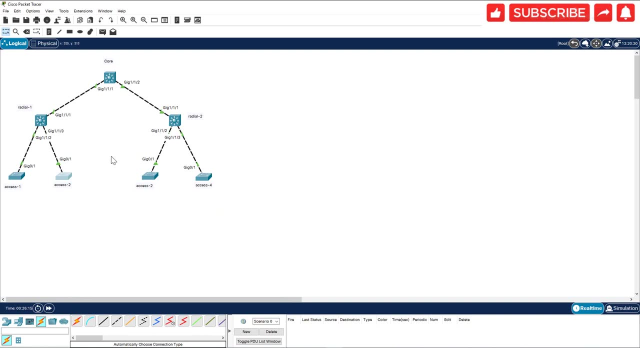 dash 2.. now it is access dash 2 and right, that's right, mem. so you have to do this to all the switches. so when you click on the switch, you know the name of the switch that you are working on. hope you like this video. if you like this.